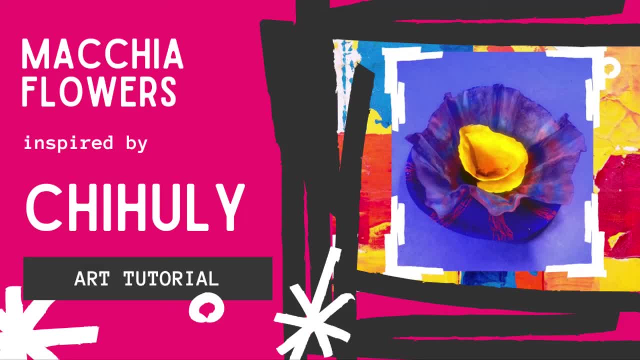 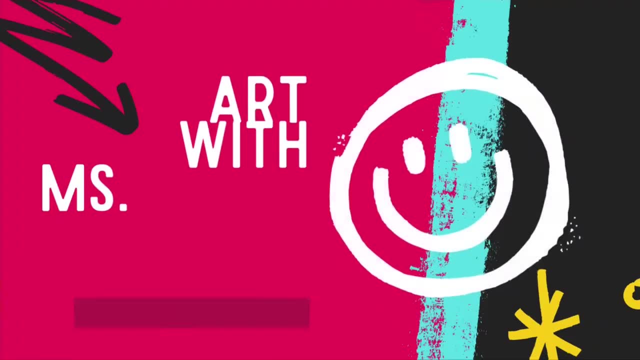 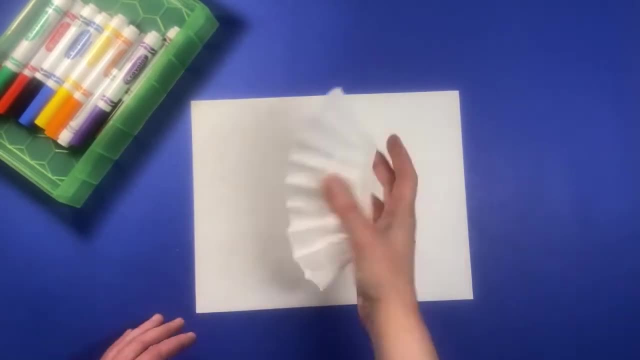 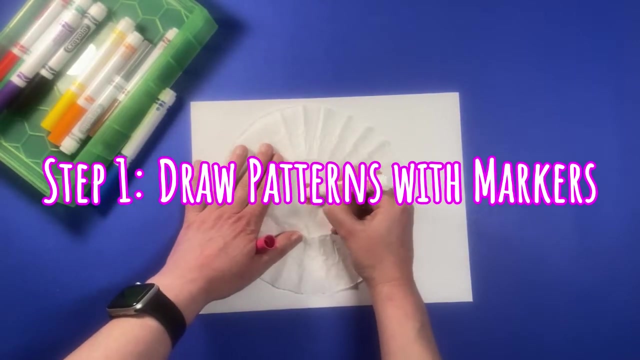 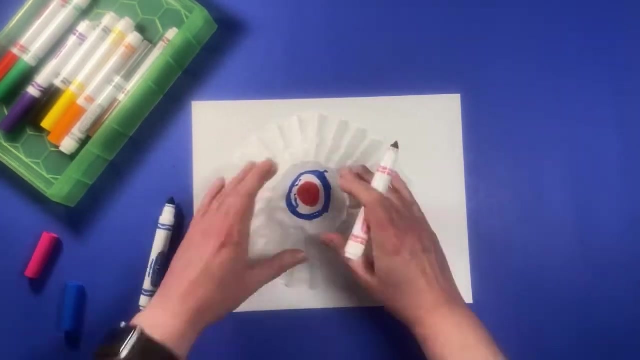 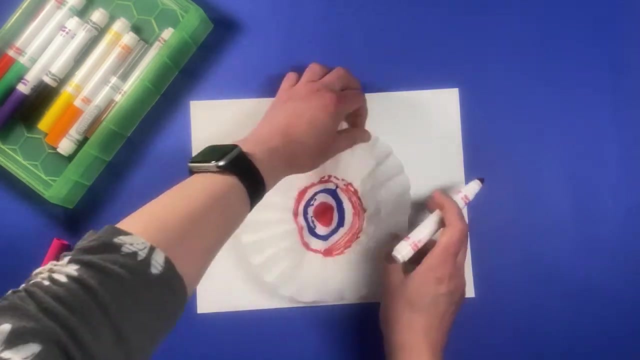 Hello everyone. it's Ms Gibbs. Today we are going to make makiyas inspired by Dale Chihuly. We are going to start with drawing patterns with markers, like you see that I'm doing here, And we're going to do some alternating patterns. So I'm just doing pink and then blue, and then pink and some more blue. 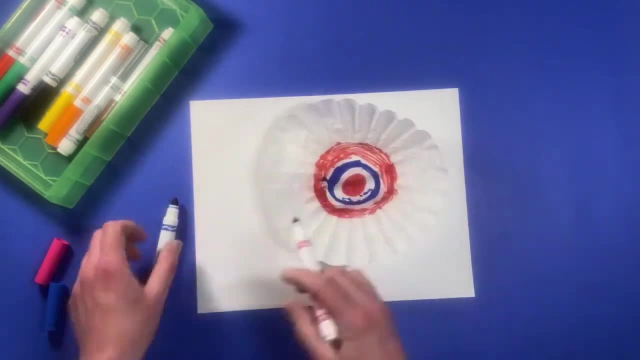 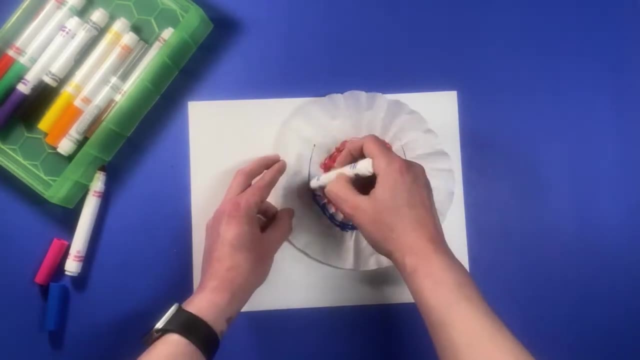 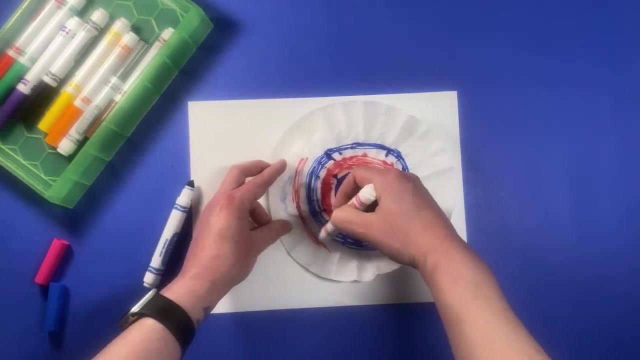 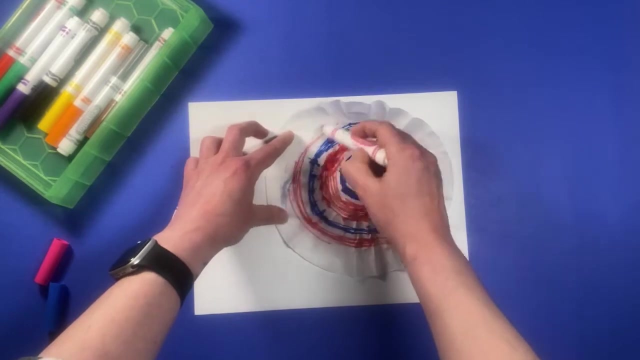 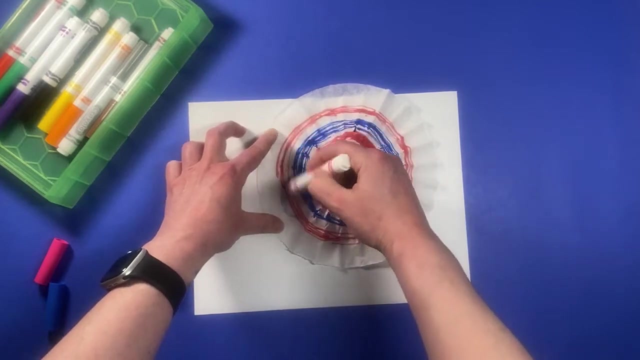 Be careful while you are using the markers on these coffee filters because they will rip if you press too hard or go over the same spot too many times. So just go over it, just enough to get some color on the coffee filter. You can see if you go in one direction and just rotate the coffee filter. that seems to work pretty well. 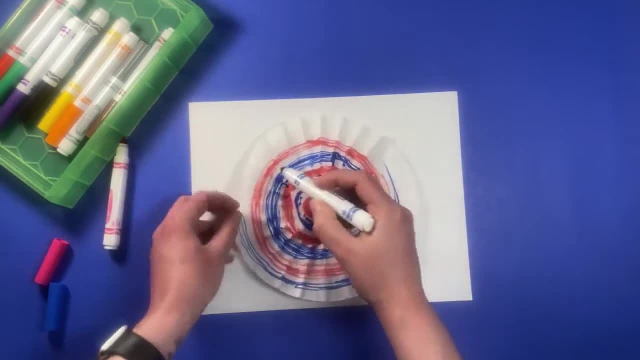 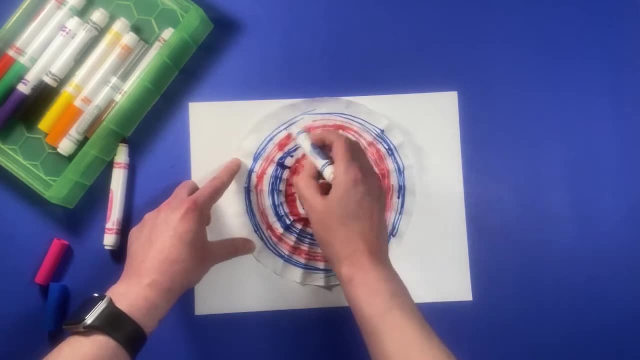 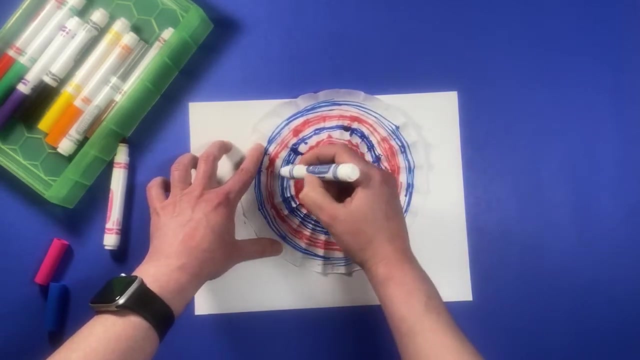 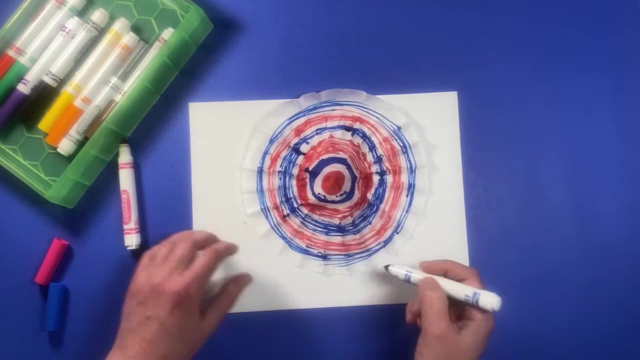 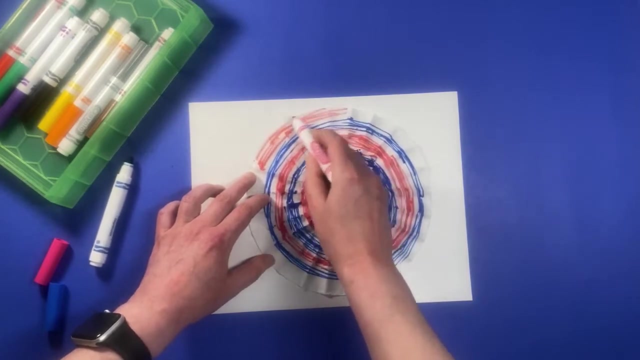 Or if you go in the other direction and just rotate the coffee filter. that seems to work pretty well. And here I'm just going back in and filling in some areas that I feel could use a little bit more color. So here I'm going to do a sign that goes right on in the center of the flower. 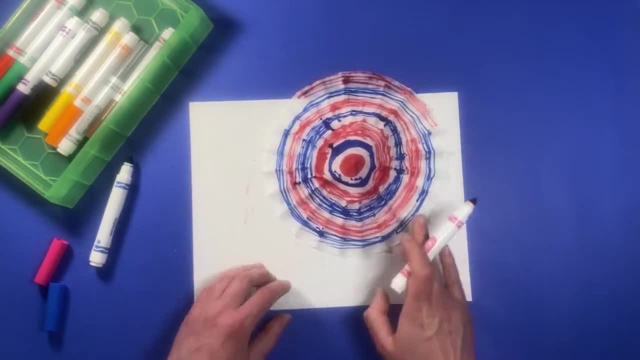 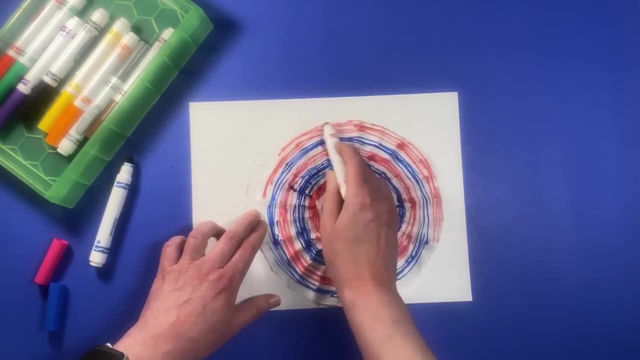 And I'm just going to take the green and I'm going to trace this all the way down the center of the flower so that it looks clearly, And then make a couple of more signs that are in the center of the flower. So I'm just going to take the green and I'm just going to add these little dots on the center of the flower, like so: 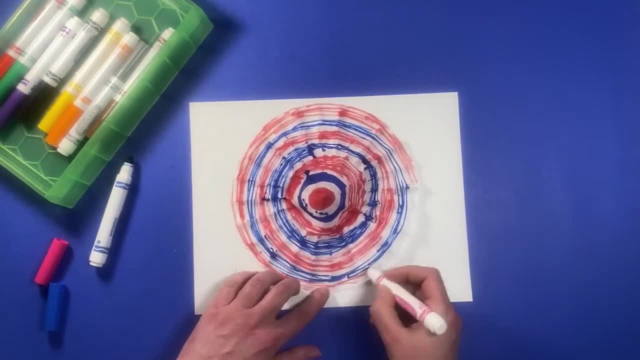 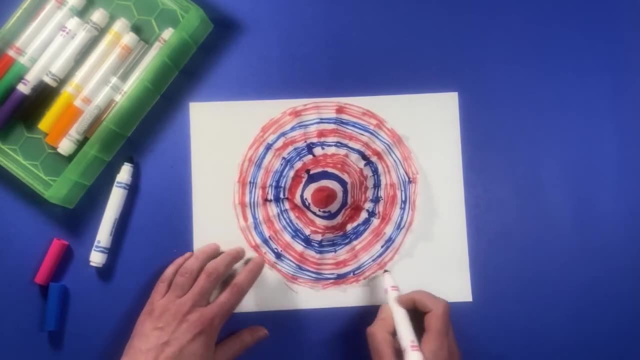 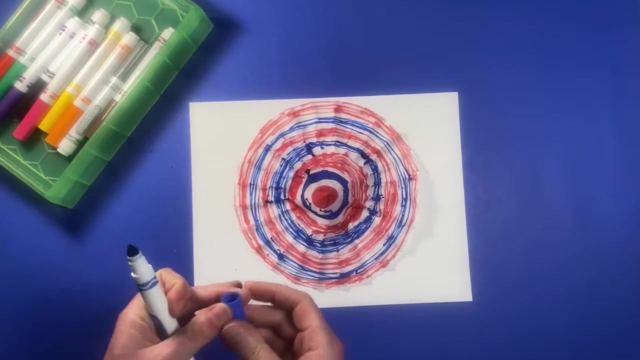 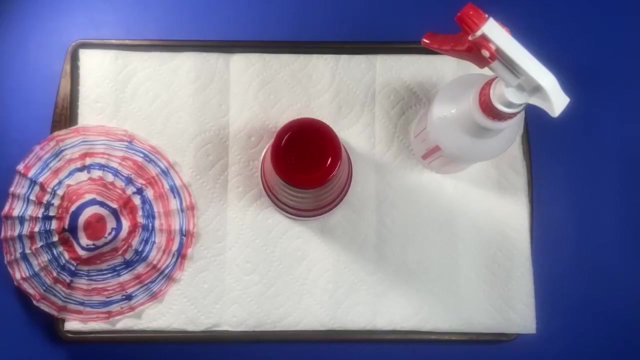 And this makes all of the colors look more natural And this will make the color more visible and this will make the color look a little more static. So it's kind of like a circle, And that's how I was doing it. and remember to put the caps back on your markers. our next step: we are going. 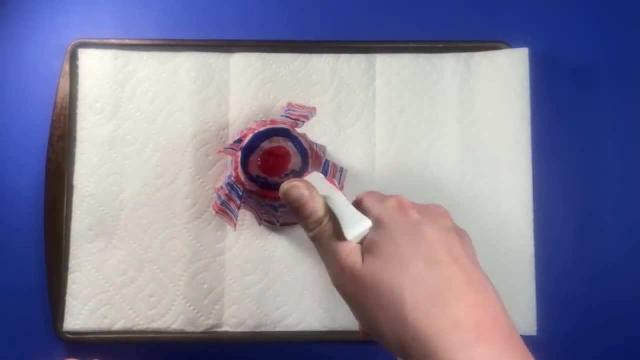 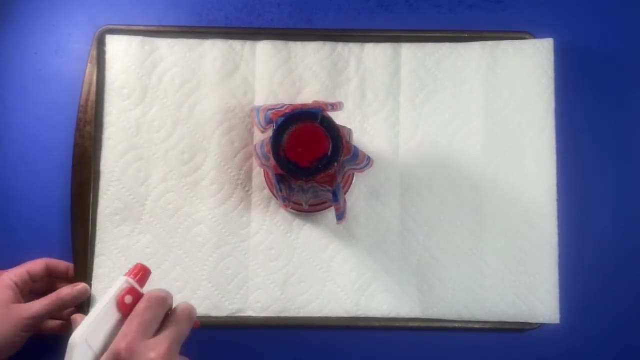 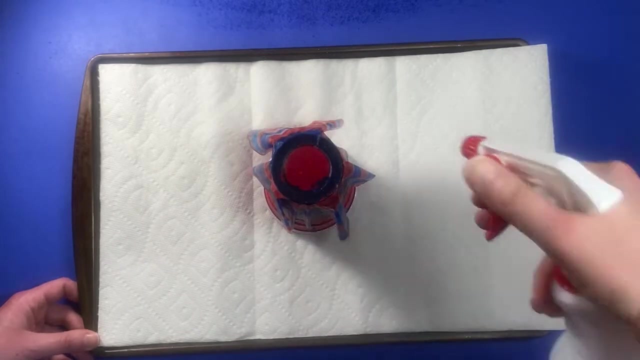 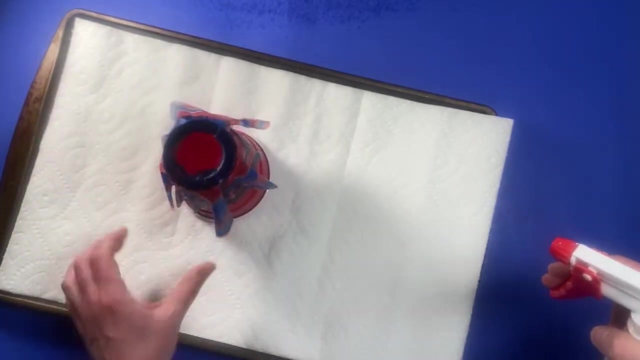 to put the coffee filter on top of a cup and spray it with some water. notice, I am not drenching it with water, I'm just giving it a few spritzes. you can see the color will start to run down the sides, but if we add too much water it's going to end up completely. 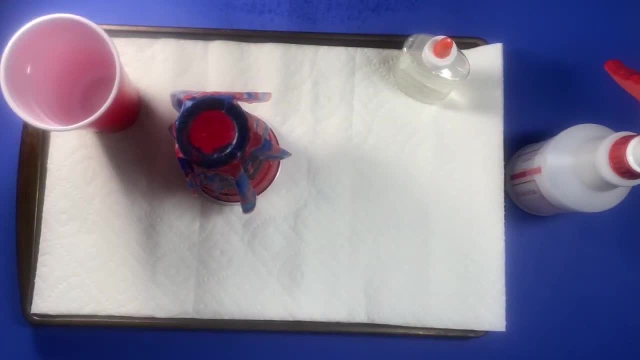 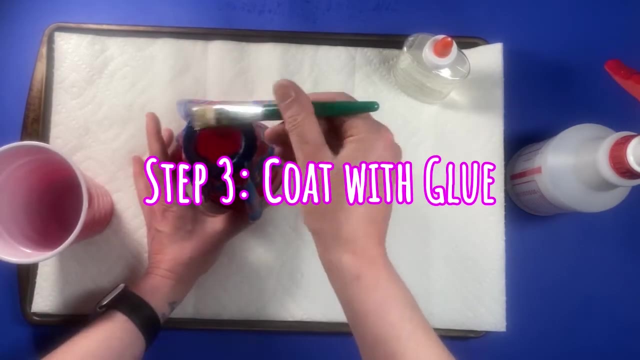 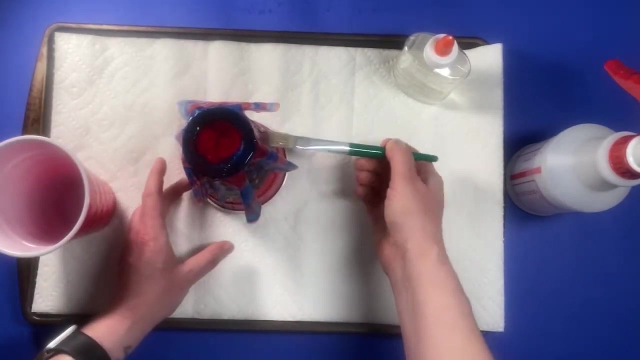 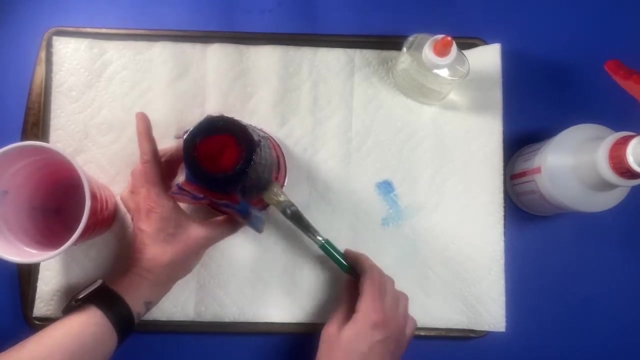 washing out the color, and that's something that we don't want. now I am coating the makia with glue and I'm just painting it on lightly, and this is going to help it keep its form when it dries. be gentle when you're applying the glue, because this is delicate and we don't want it to rip. 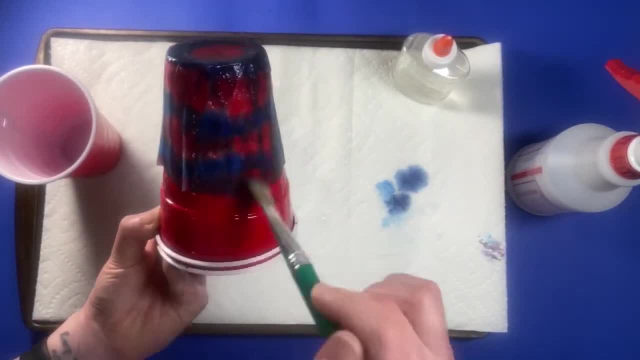 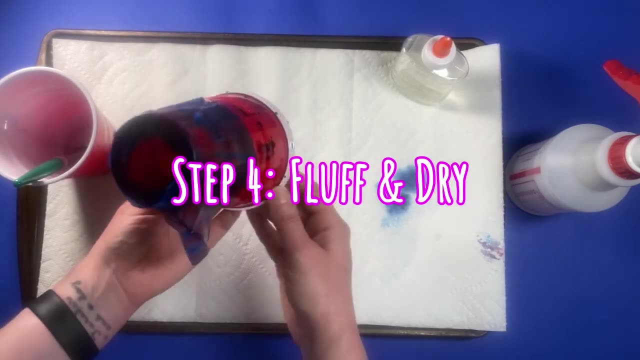 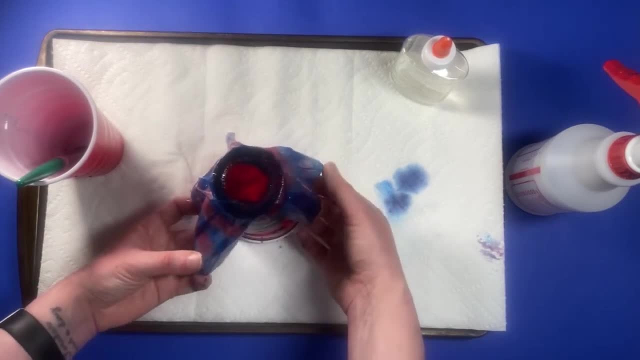 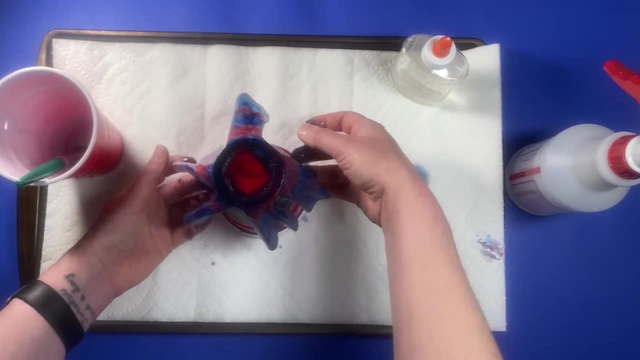 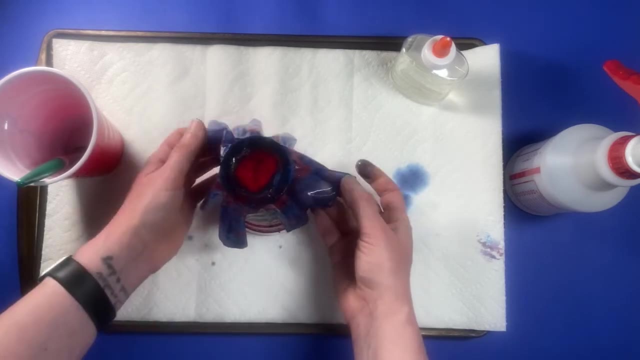 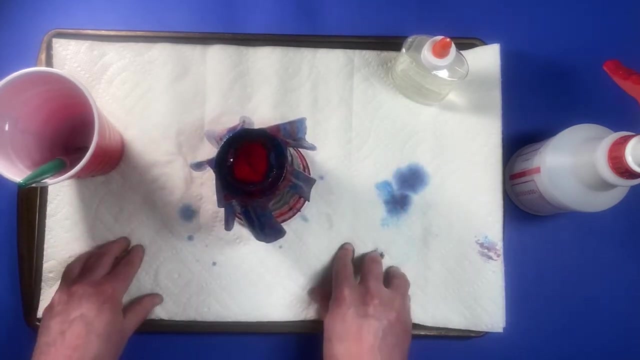 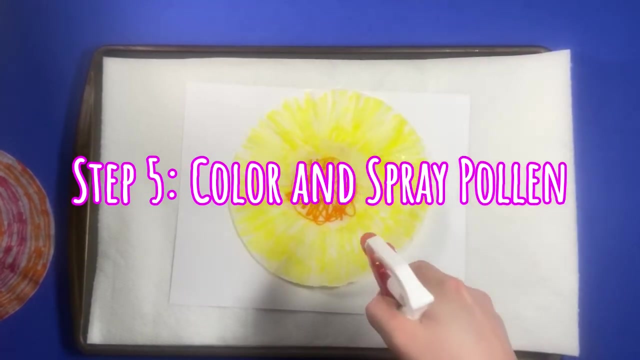 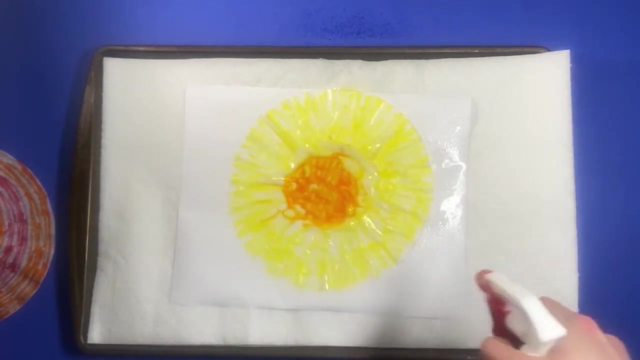 sit wherever it falls. It is going to take a bit of time for that to dry, So in the meantime we can color and spray something for the inside of the makia so it looks like a flower. And what I did here was I colored a coffee filter using orange and yellow, and that's. 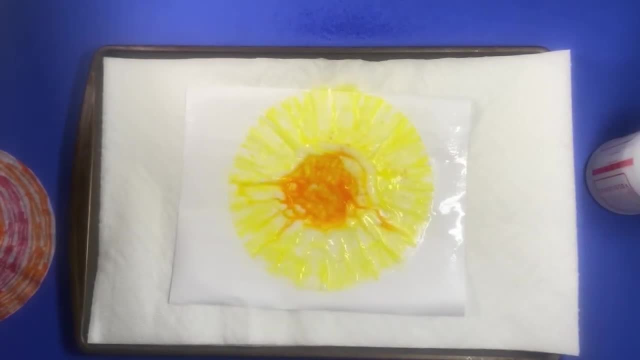 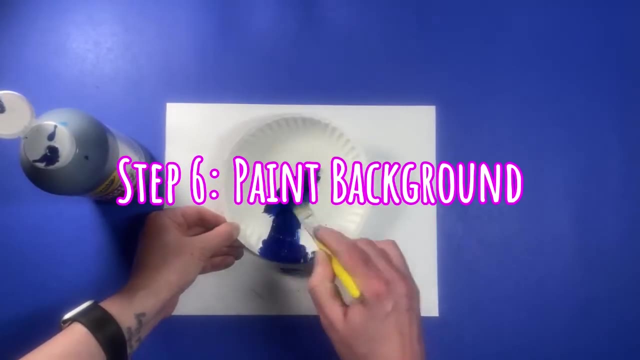 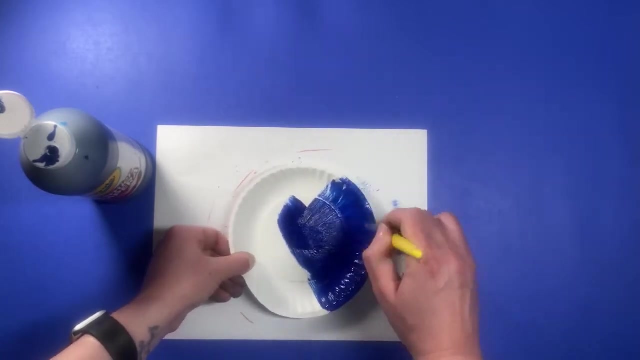 going to be some pollen for the inside. I'm just going to lay it flat to dry. Here I am painting a paper plate for the background because I thought it would be neat to have it mounted on something so we can hang them up, And I chose the same colors. 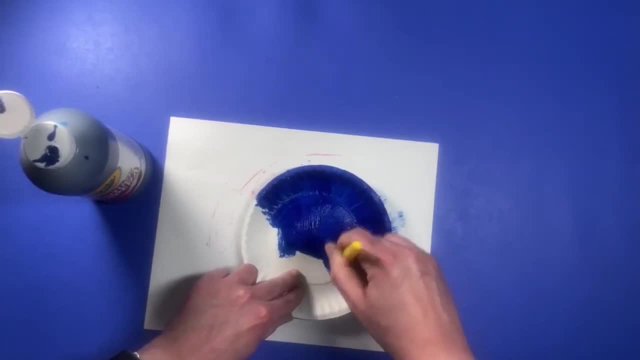 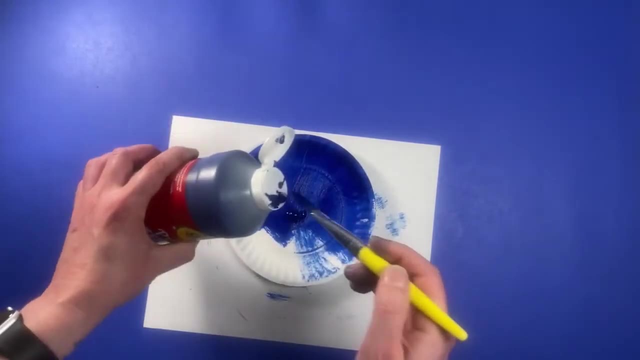 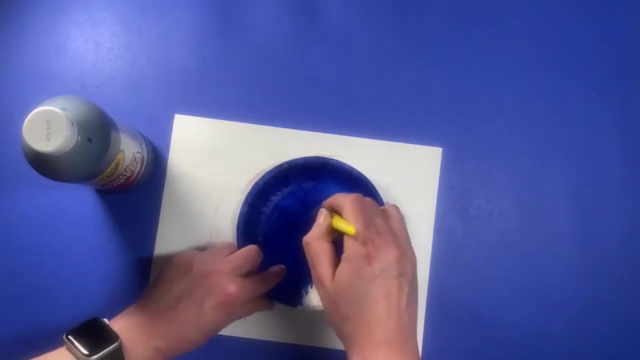 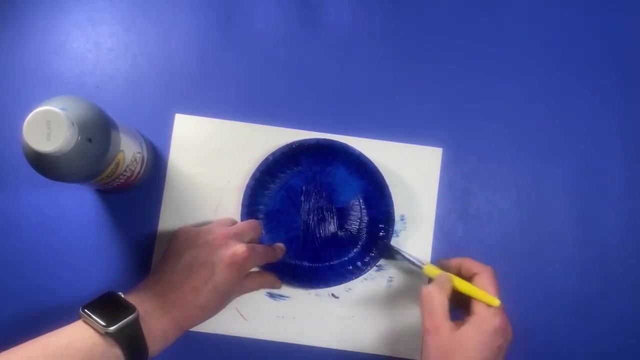 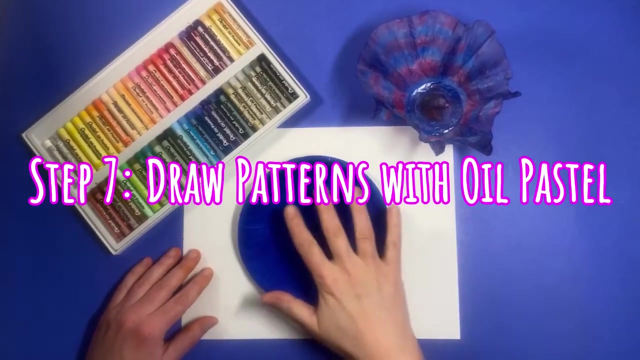 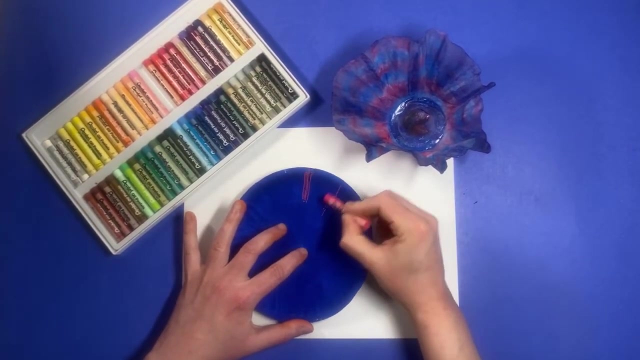 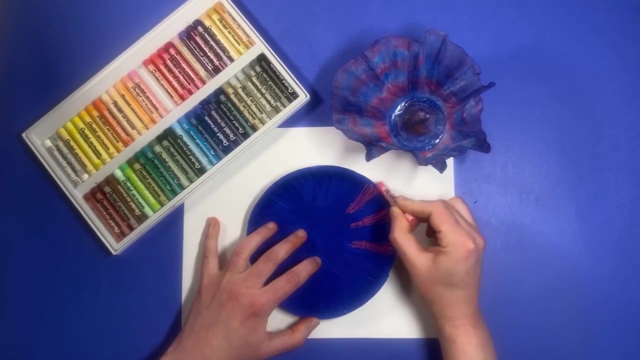 That I used for the makia. Now, after that has some time to dry, we can draw some patterns on the background, And again I chose colors that go with the makia that I made. So I have a blue background and I am doing some pink stripes on it. 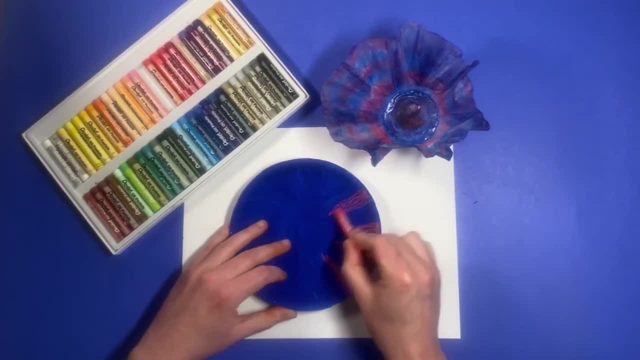 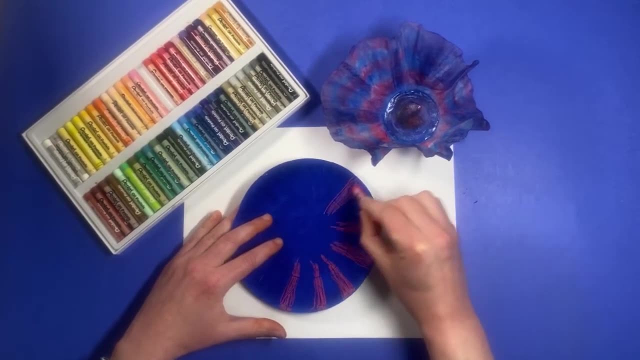 It doesn't have to be stripes, It could be whatever you want, But our goal here is to do a pattern. So, since I have pink blue, pink blue, that is the AB, The pattern that we learned about in math. 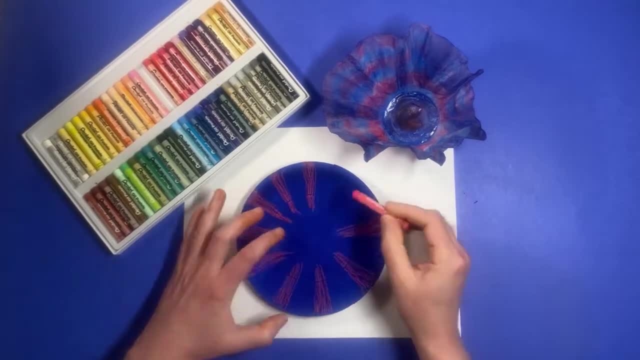 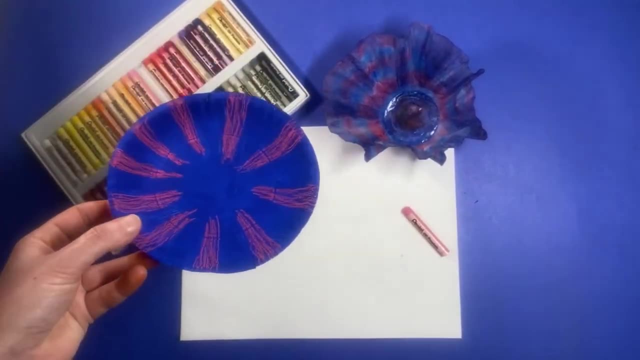 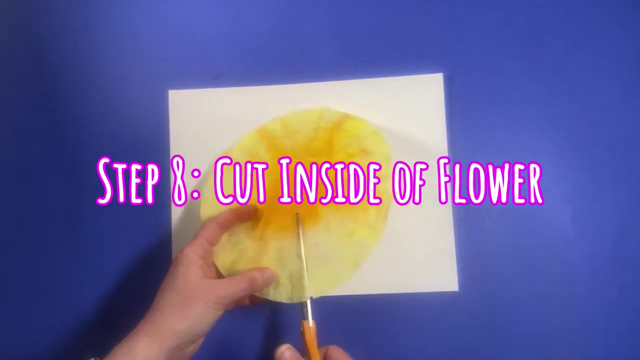 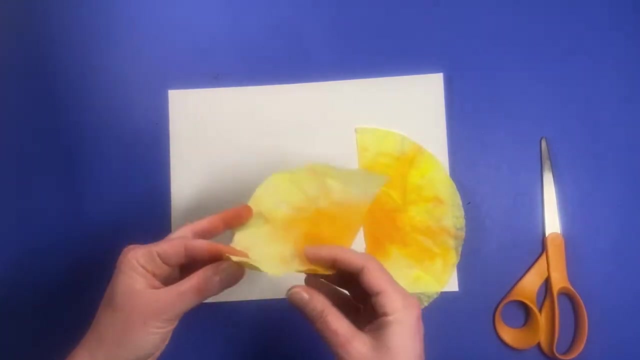 So that's what I'm going to repeat here. That's what I did on the makia. Now we are going to cut the coffee filter that's dry to make the inside pollen part of our flower And It's going to be like a mini makia shape here. 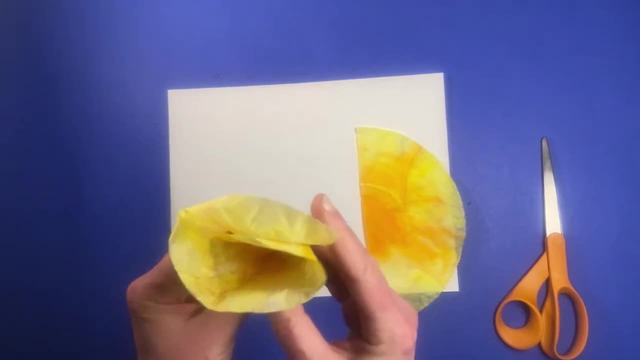 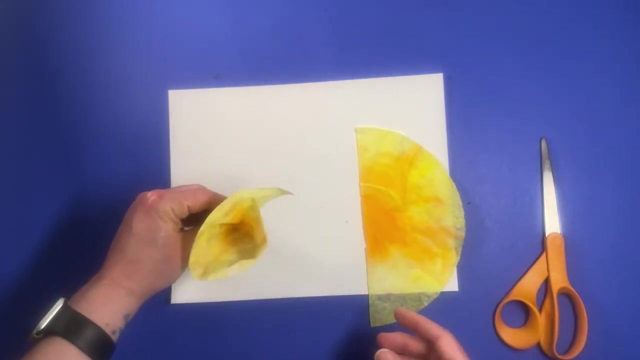 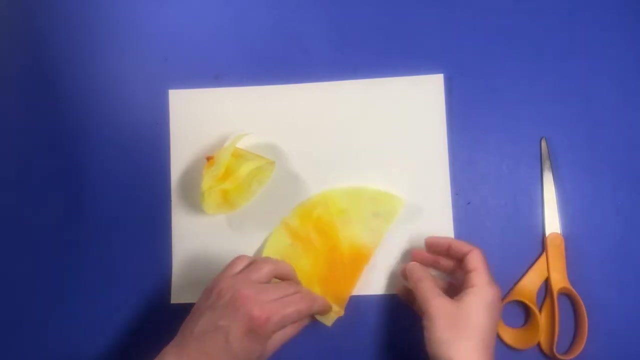 I am just kind of overlapping it and then pinching it at the bottom, So I have a circular type shape here That you can also do with tissue paper. I didn't have any tissue paper when I did this at home, So I decided to make my own.